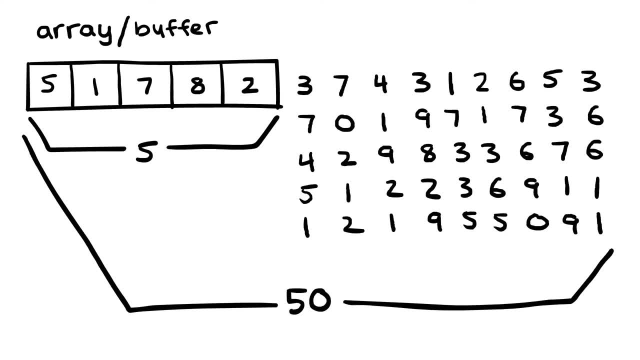 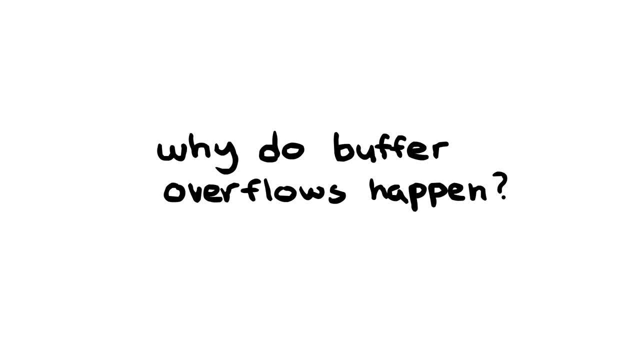 put six numbers in there, put 10 numbers in there, put 50 numbers in there, you get the idea. Let's talk about why these overflows are even allowed to happen in the first place. Clearly, putting six numbers into an array that holds five numbers is not an operation that we should allow, And 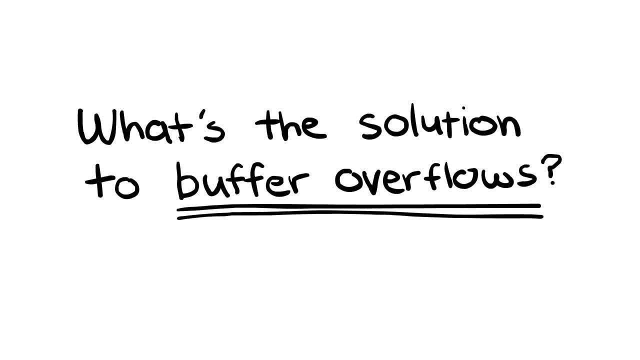 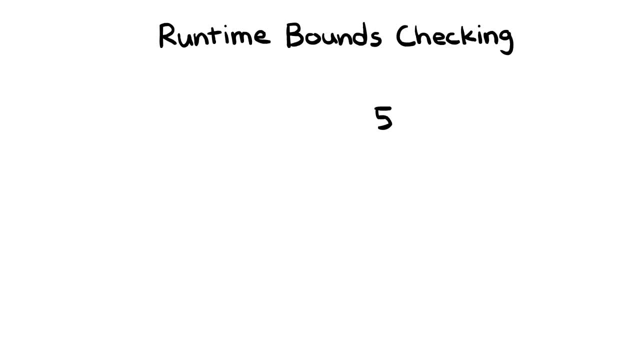 so what's the solution to buffer overflows? The solution we're looking for is known as runtime bounds checking. With runtime bounds checking, every time we want to add a number to our array, there's code behind the scenes that will check if the array has enough room to fit our new number. 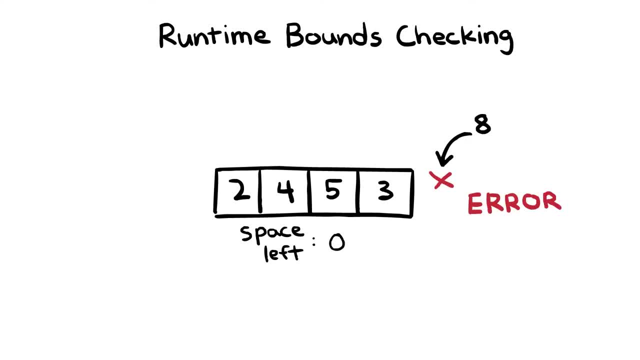 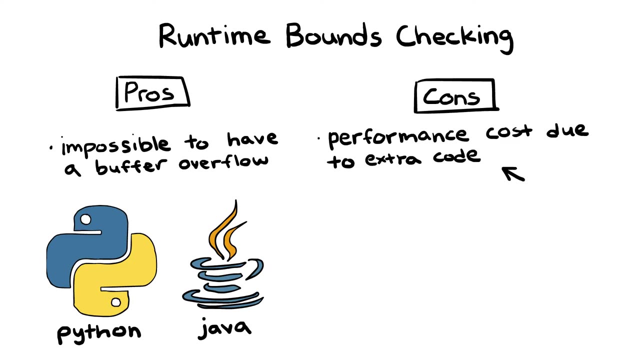 If there's no room in the buffer, the insertion will not happen and an error will be reported. The upside to doing this is that it makes it theoretically impossible to have a buffer overflow. This tremendous upside has been adopted by many mainstream programming languages like Python and Java. However, there is a performance cost for 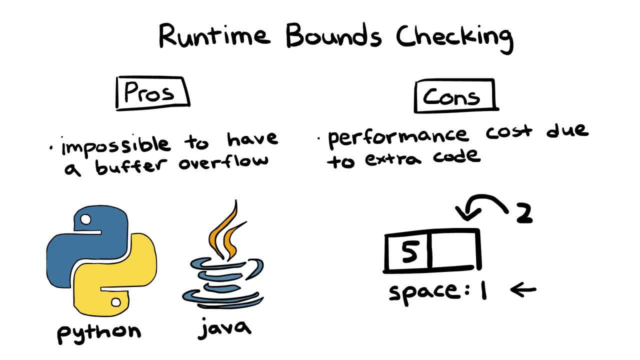 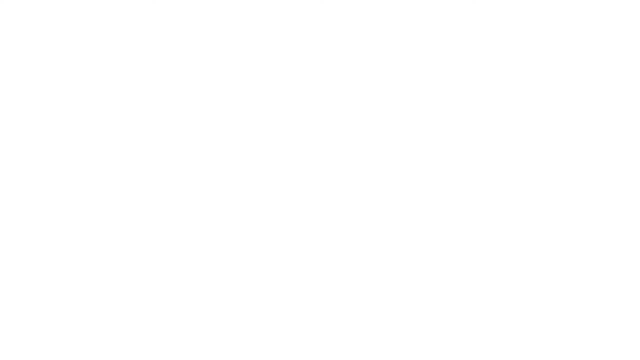 the extra code we're running every time we want to insert an element into the array And thus programming languages like C and C++ have chosen not to use runtime bounds checking by default. These languages will be at the center of our discussion, since they're the only languages in 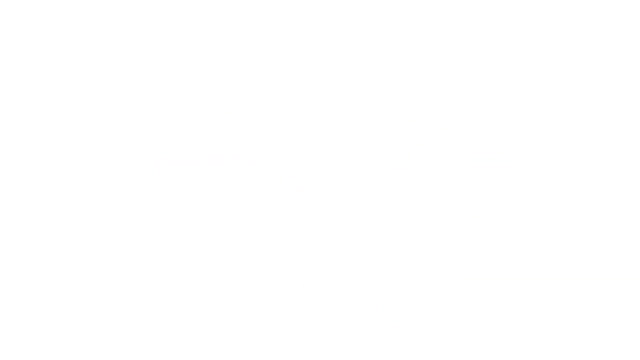 which a buffer overflow is even possible. Buffer overflows are classified as software bugs And there's a case for arguing that programmer error is the only way to get a buffer overflow. However, there are many cases where buffer overflows have been discovered in software that has been in use for decades. 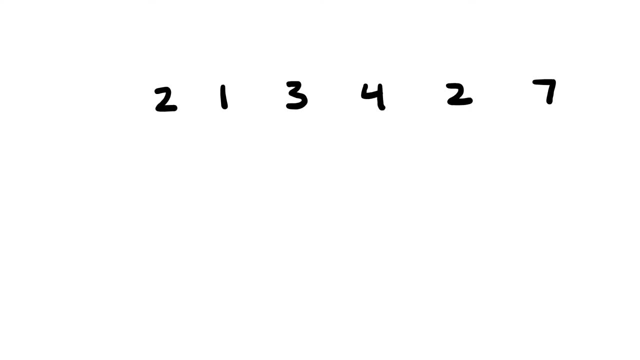 There are many cases where buffer overflows have been discovered in software that has been in use for decades. After all, no one in their right mind would try to put six numbers in an array that only holds five numbers. Well, it's not as simple as just not making mistakes as a programmer. Oftentimes, 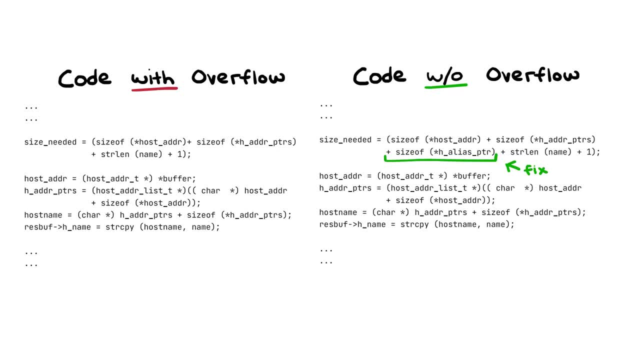 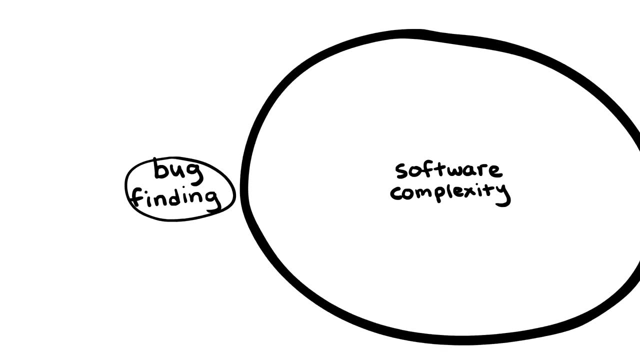 buffer overflows are notoriously difficult to find, and history has shown time and time again that software complexity has quickly outgrown our ability to catch and deal with these kind of bugs efficiently. There are many cases where buffer overflows have been discovered in software that has been in use for decades. 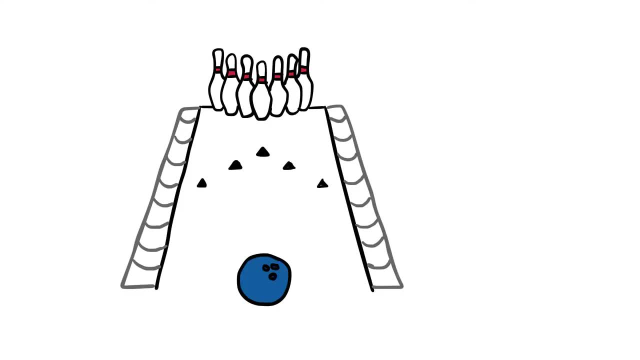 I like to compare the entire situation to bowling, where runtime bounds checking is like the bumpers. Sure, you could say that without the bumpers, it's the bowler's fault if they go to the ball, But why not remove that option entirely, For most bumpers would probably improve their score by. 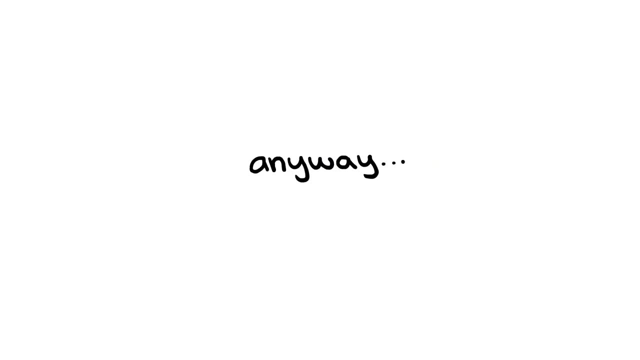 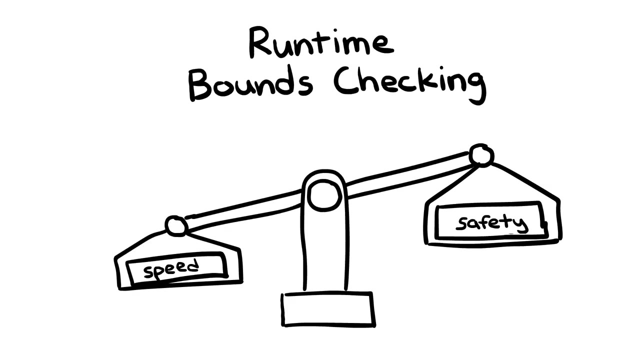 getting rid of the possibility for a gutter ball. Anyway, the point I want to make is that runtime bounds checking is one possible solution to buffer overflows, but it is a choice that has trade-offs. Now that we've covered why buffer overflows can happen, 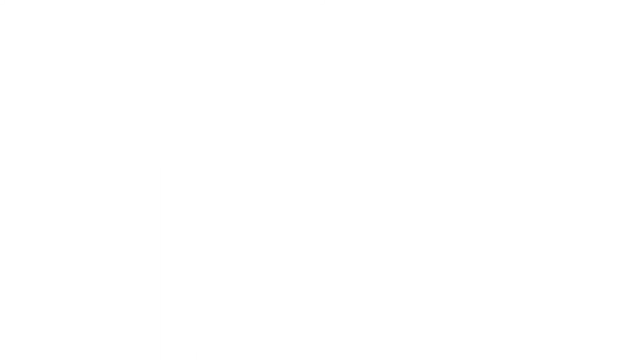 let's talk about the damage they can do. Often, the buffers we're talking about are local variables, meaning that they're going to be put in an area of memory called the stack. Remember when I said at the beginning that there was some important information that could be. 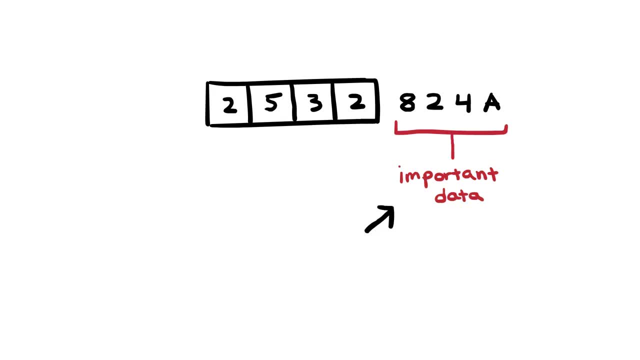 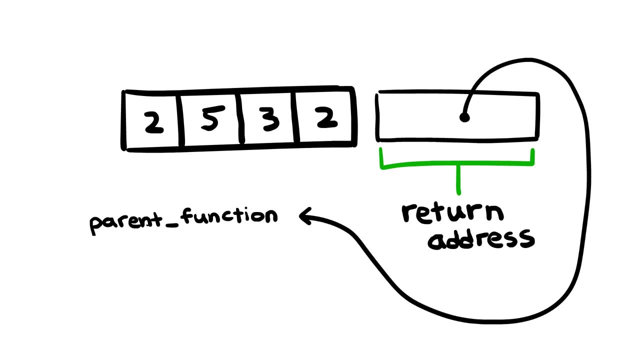 overwritten by a buffer overflow. Well, that information I was talking about is known as a return address. The return address represents the location and code that we're going to go back to after we're done with the current function. Typically, a user cannot interact with, or even see the return address. 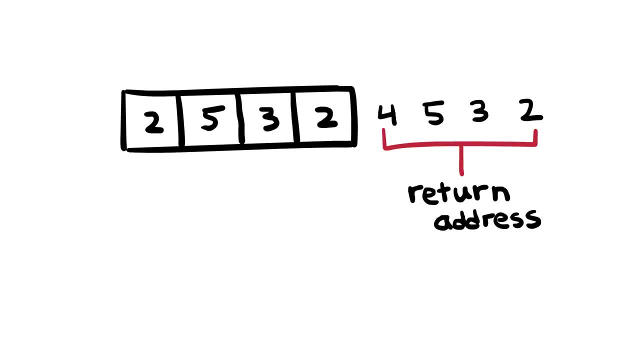 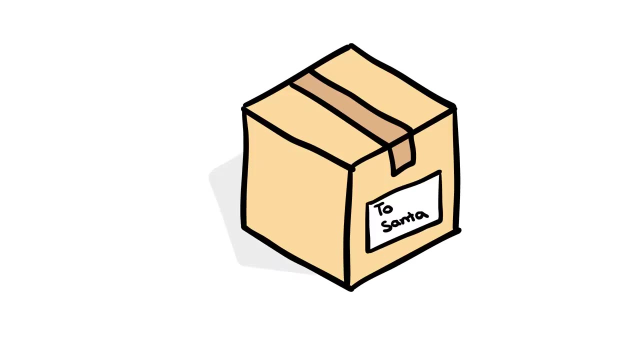 However, with a buffer overflow there's a chance that the return address will get overwritten. Normally a buffer overflow would result in a program crash because the overwritten return address probably doesn't point to a valid program instruction. It's kind of like a package addressed to a place that doesn't exist. 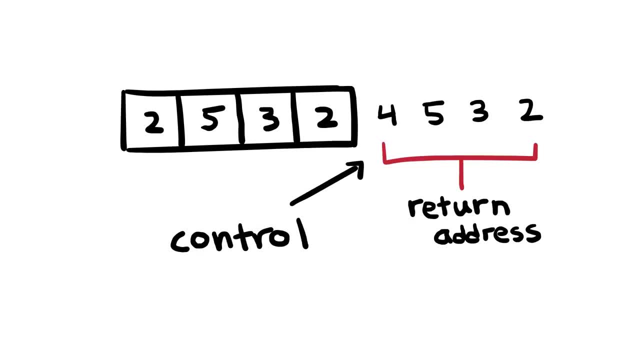 But if someone were able to control the contents of the buffer overflow, they might be able to carefully choose a return address that points to a place in code that they want to execute. This type of user-controlled buffer overflow can happen when a program tries to take user input. 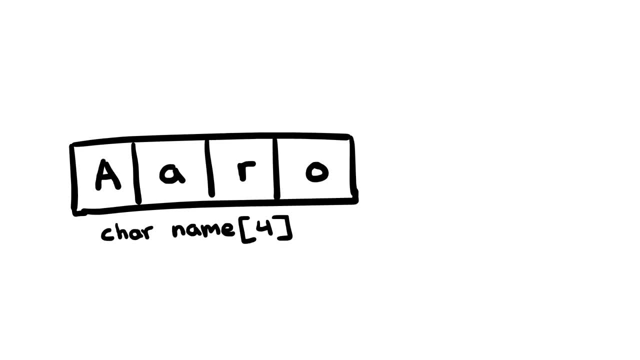 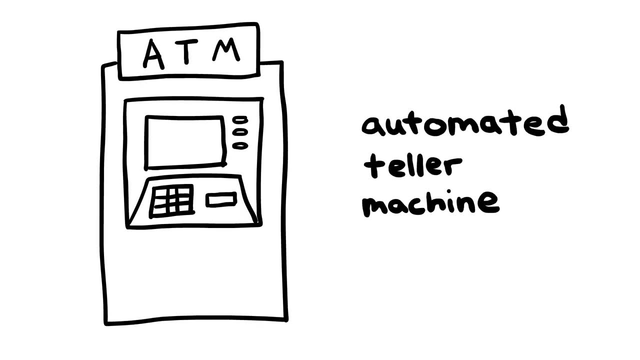 like a user's name but forgets to check to make sure that the buffer is large enough to hold the given name. To show you what I mean, consider an ATM. There's probably a function somewhere in the ATM code that dispenses money. 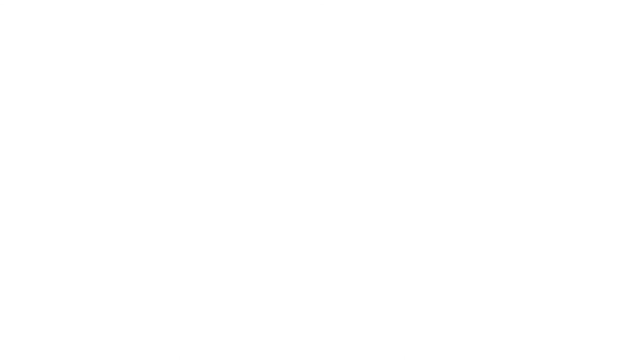 since that's one of its core jobs. If there's a buffer overflow in the ATM when it prompts us to type in our name, if we type in just the right name, we can overwrite the return address of the getName function with the address of the dispenseMoney function. 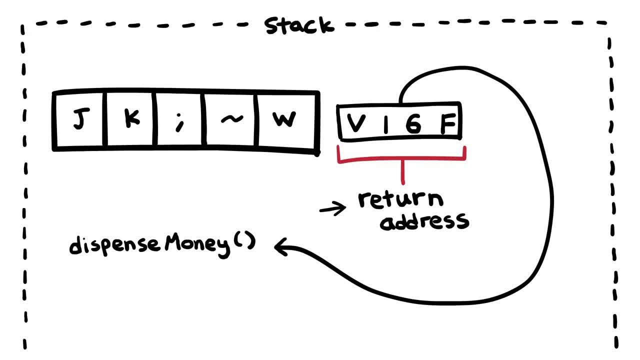 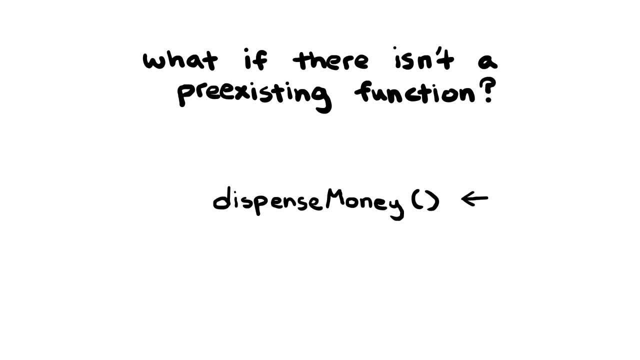 So when the ATM's done getting our name, the computer will look at the stack and start executing the dispenseMoney function And we get wildly rich. Okay, that's cool and all, but what if there isn't a pre-existing function that we want to return to, like dispenseMoney in our previous example?